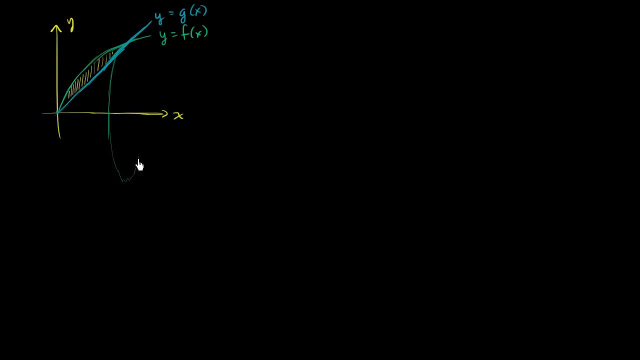 But in the way we've drawn it now, it would literally be that same truffle shape. It'd be a very similar truffle shape, where on the outside it looks like a truffle, on the outside it looks like something like a truffle, and on the inside we have carved out a cone. Obviously this visualization is very specific to the way I've drawn these functions, but what we wanna do is generalize at least the mathematics of it. 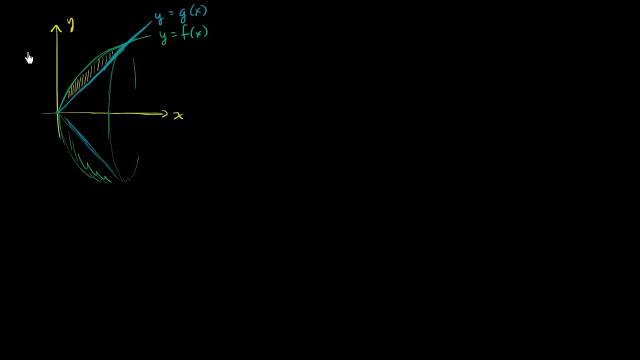 So how do we find a volume? Well, we could think of disks, but instead of thinking of disks, we're gonna think about washers now, which is essentially the exact same thing we did in the last video mathematically, but it's a slightly different way of conceptualizing it. So imagine, imagine a, imagine taking a little chunk between these two, between these two functions, just like that. 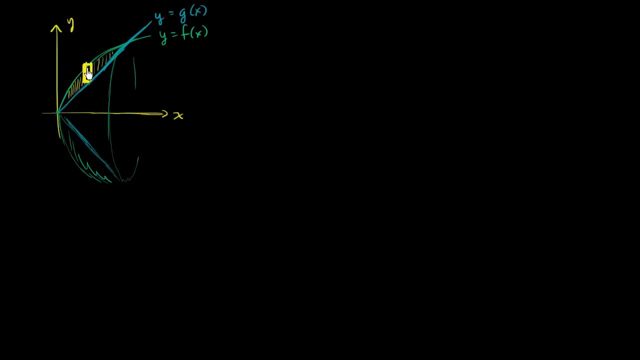 What is going to be, what is going to be the width of this chunk? 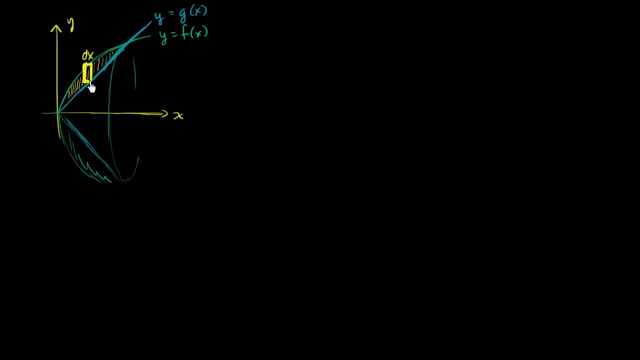 Well, it's going to be equal to dx, and let's rotate that whole thing around the x-axis. So if we rotate this thing around the x-axis, we end up with a washer. 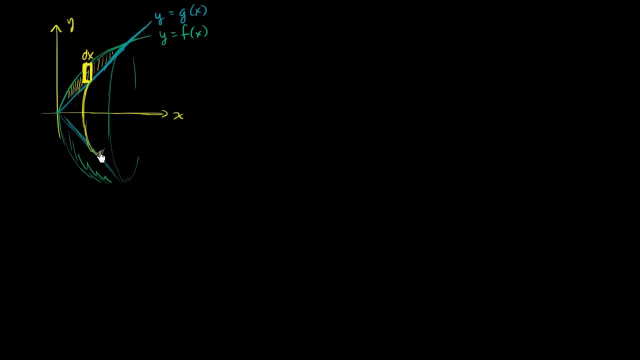 That's why we're gonna call this the washer method. And it's really just kind of the disk method where you're gutting out the inside of a disk. 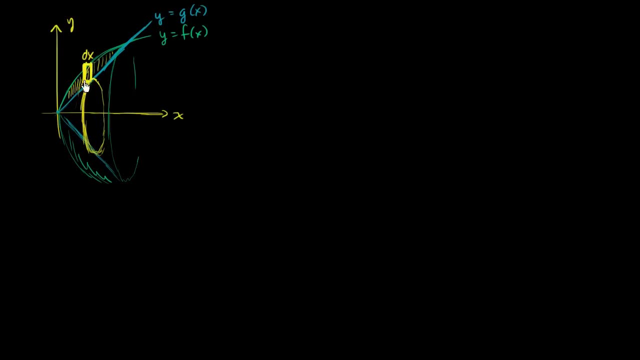 So that's the inside of our washer, and then this is the outside of our washer. 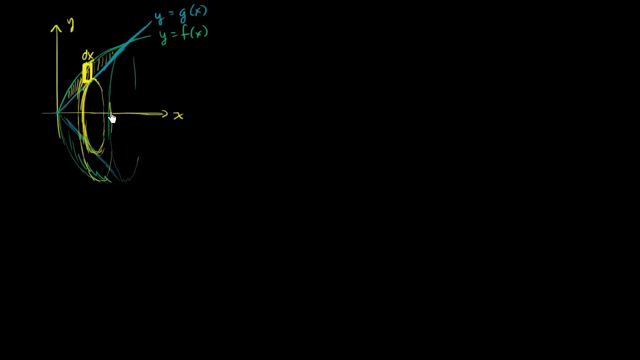 Outside of our washer looks something like, looks something like that. Hopefully that makes, that makes sense. 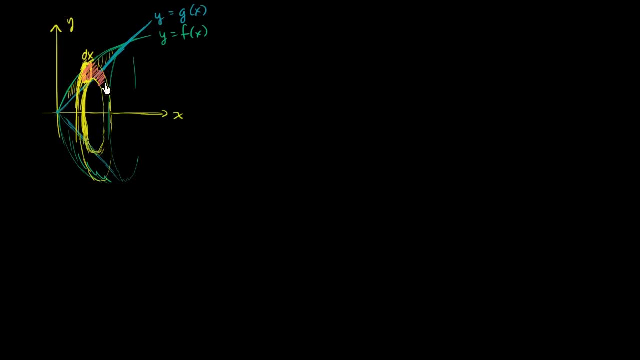 And so the surface of our washer, the surface of our washer looks something like that. 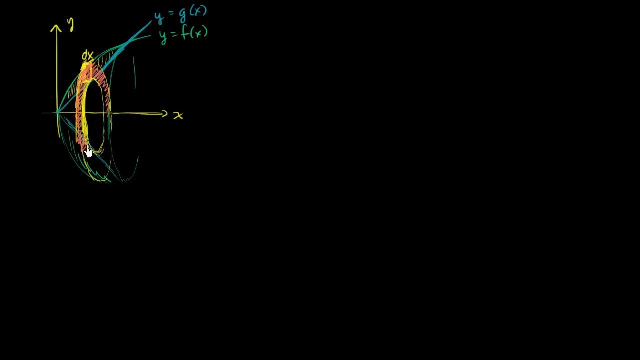 I know I could have drawn this a little bit better, but hopefully it serves the purpose so that we understand it. 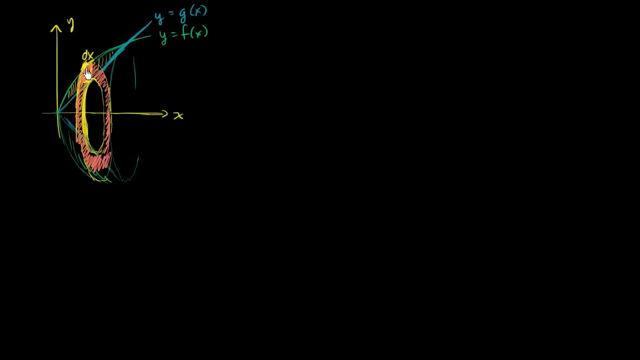 So the surface of our washer looks something like that, and it has depth of dx. It has depth dx. 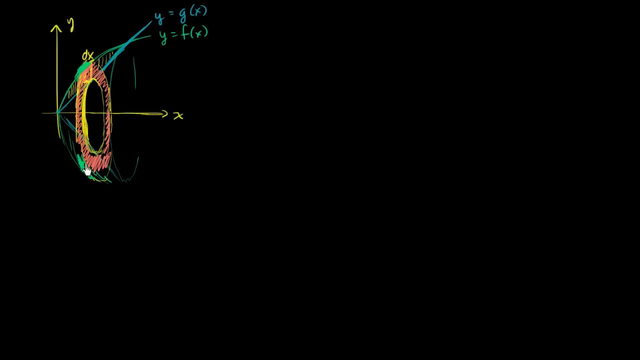 So let me see how well I can draw this. So depth dx, that's the side of this washer. 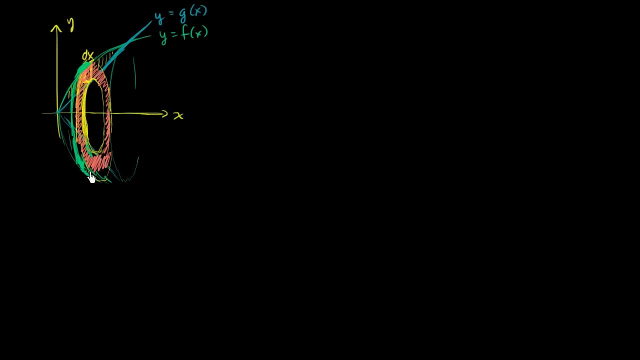 So a washer you can imagine is kind of a gutted out, it's a gutted out coin. It's a gutted out coin. 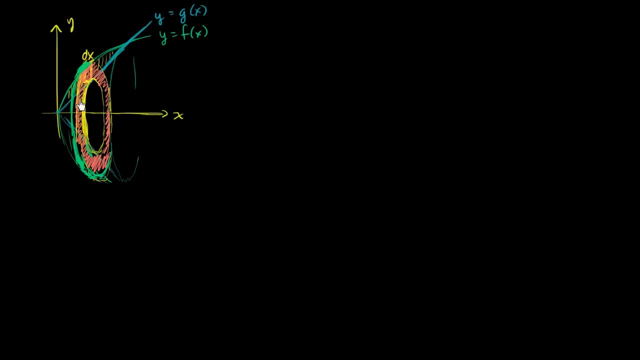 So how do we find the volume? Well, once again, if we know the surface, if we know the area of the face of this washer, we can just multiply that times the depth. 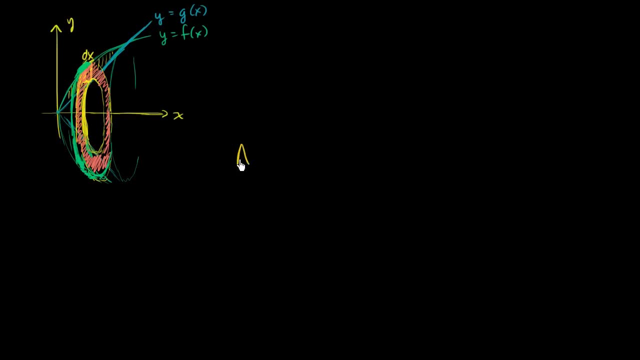 So it's gonna be the area of the face of the washer. So the area of the face of the washer, well, it could be the area if you had, if it wasn't gutted out, and what would that area be? 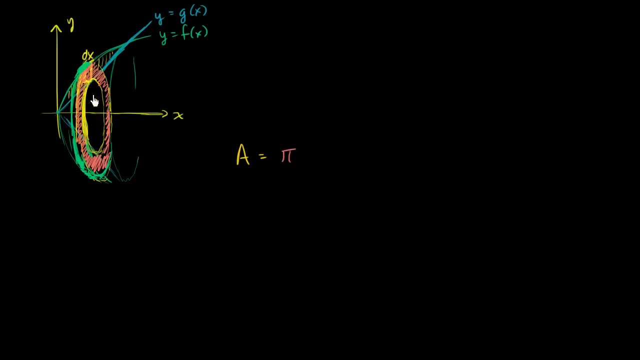 Well, it would be pi times the overall, the outside radius squared. It would be pi times the outside radius squared. 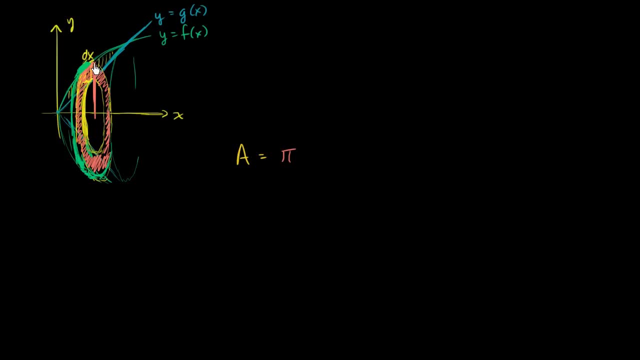 Well, what's the outside radius, the radius that goes to the outside of the washer? Well, that's f of x. 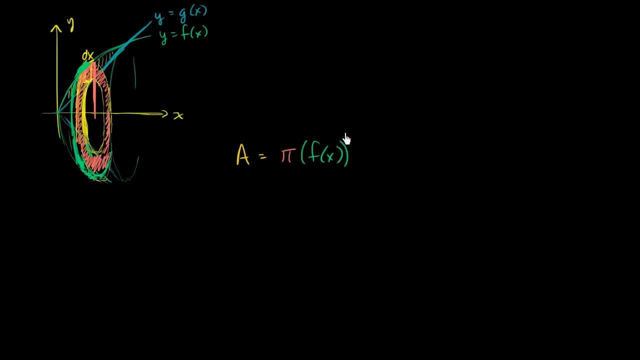 So it's gonna be f of x and we're just going to square that. 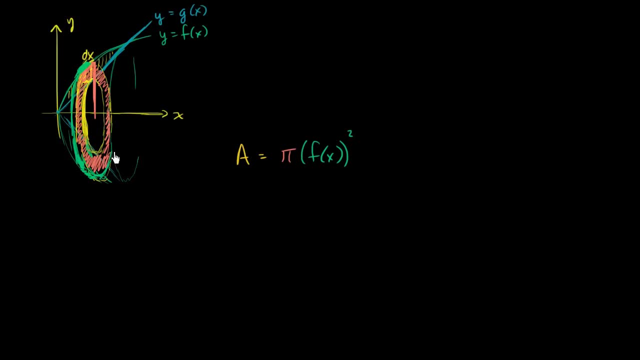 So that would give us, this expression right over here would give us the area of the entire face if it wasn't a washer, if it was a coin. 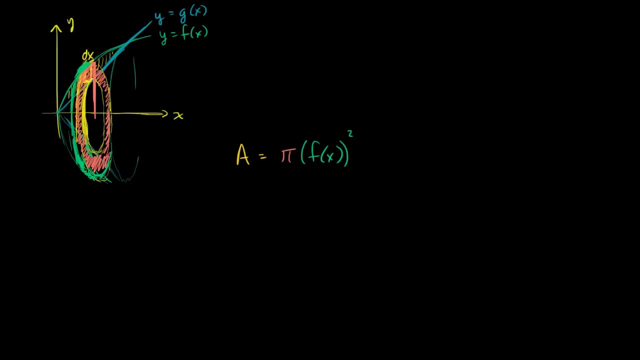 But now we have to subtract out the inside. So what's the area of the inside? What's the area of the inside? This part right over here. Well, we're gonna subtract it out. 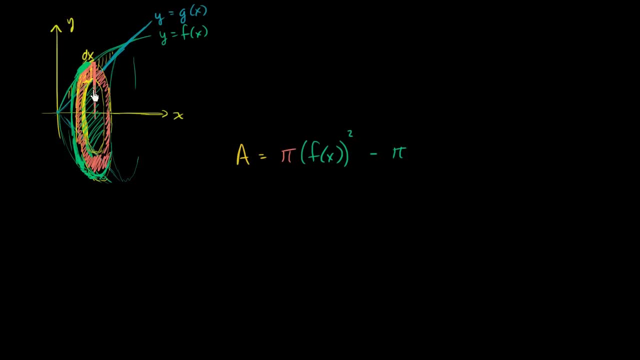 It's going to be pi times the radius of the inside squared. The radius of the inside squared. 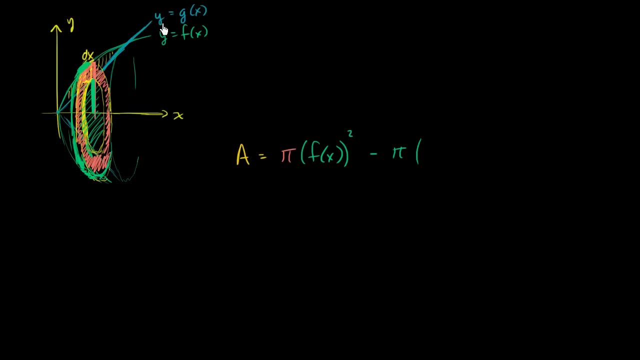 Well, what's the radius of the inside squared? Well, the inside in this case is g of x. 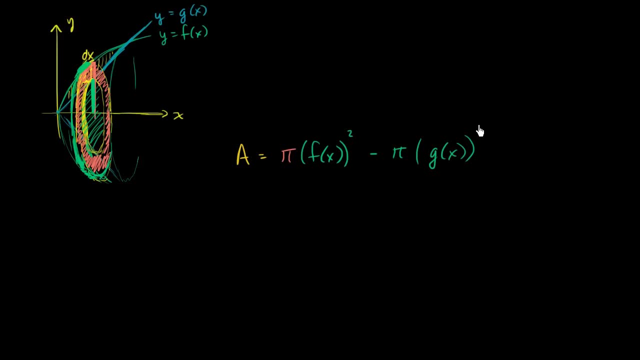 It's going to be pi times g of x squared. That's the inner function, at least over the interval that we care about. 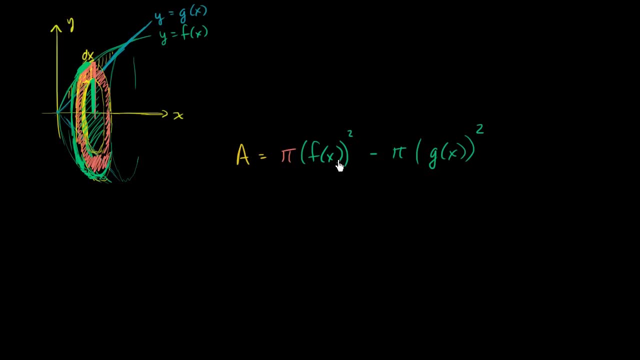 So the area of this washer, we could just leave it like this or we could factor out a pi. 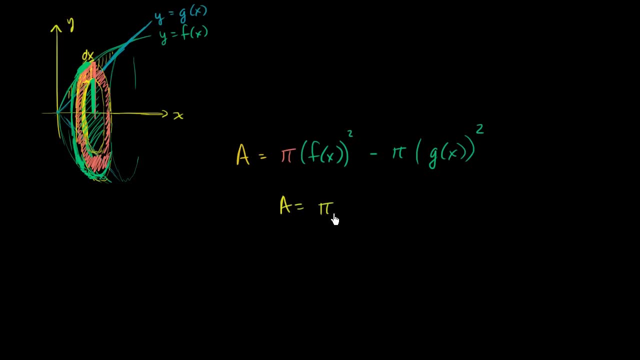 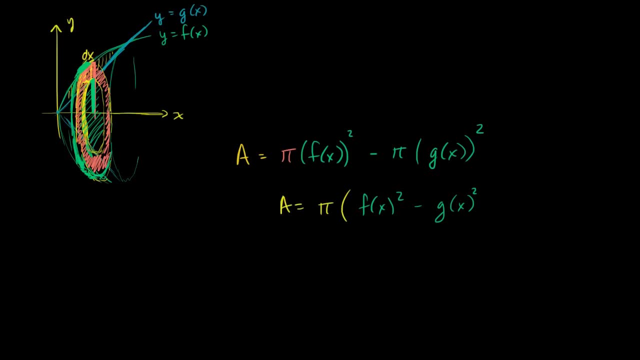 And then if we want the volume, put that in that same yellow. If we want the volume of this thing, we just multiply it times the depth of each of those washers. So the volume of each of these washers are going to be pi times, pi times f of x squared minus g of x squared. 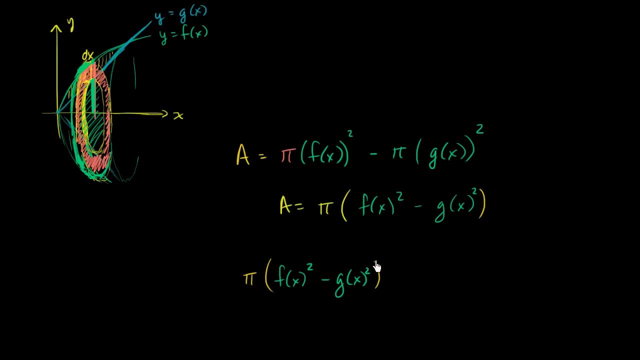 The outer function squared over our interval minus our inner function squared over the interval and then times our depth. 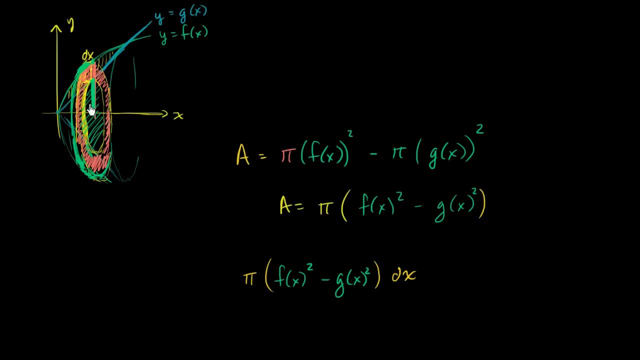 That'd be the volume of each of these washers. Now, and that's going to be defined at a given x in our interval. But for each x at this interval, we can define a new washer. So there could be a washer out here and a washer out here. So we're going to take the sum of all of those washers and take the limit as we have smaller and smaller depths and we have an infinite number of infinitely thin washers. 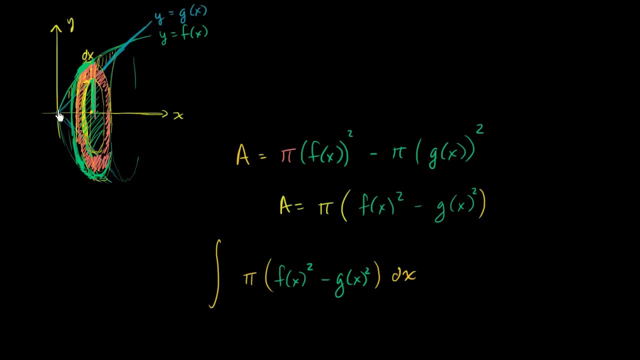 So we're going to take the integral over our interval from where these two things intersect, the interval that we care about. 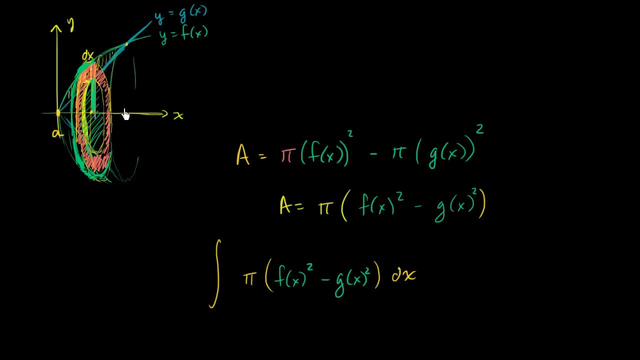 It doesn't have to be where they intersect, but in this case, that's what we'll do. So let's say x equals a to x equals b, although it could have been from, this could have been a, that could have been b, but this is our interval. 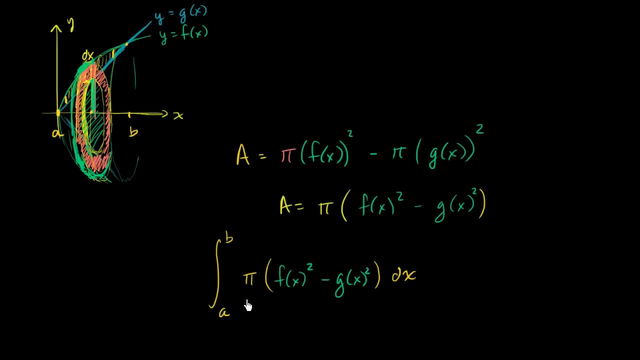 We're saying in general terms from a to b. And this will give our volume. This right over here is the volume of each washer and then we're summing up all of the washers and taking the limit as we have an infinite number of them. 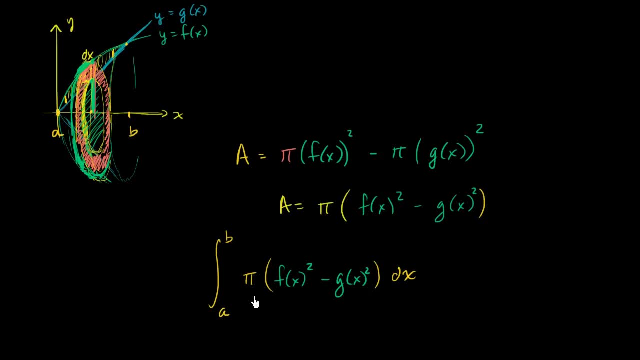 So let's see if we apply this to the example in the last video, whether we get the exact same answer. Well, in the last video, y equals g of x was equal to x and y is equal to f of x was equal to the square root of x. 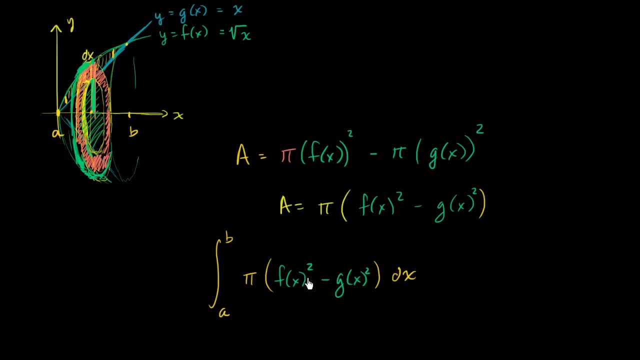 So let's evaluate that given what we just were able to derive. 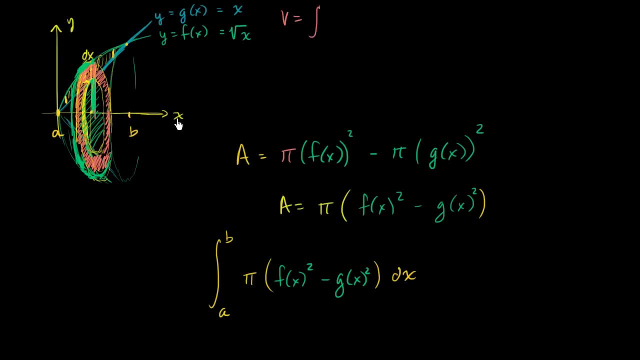 So our volume, I'll do it up here, the volume is going to be the integral. 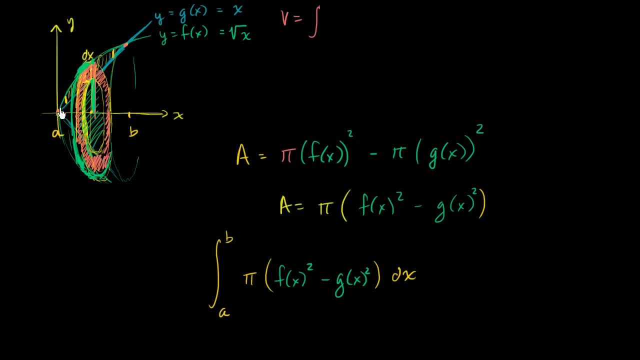 What are the two intersection points? Well, over here, once again, we could have defined the interval someplace else, like between there and there, and we would have gotten a different shape. 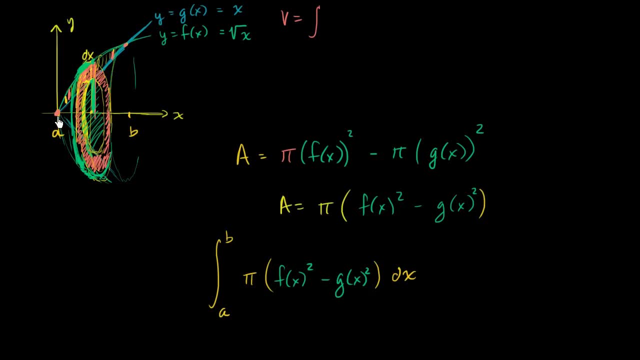 But the points that we care about, the way we visualize it, is between x is equal to 0 and x is equal to 1. That's where these two things intersect. 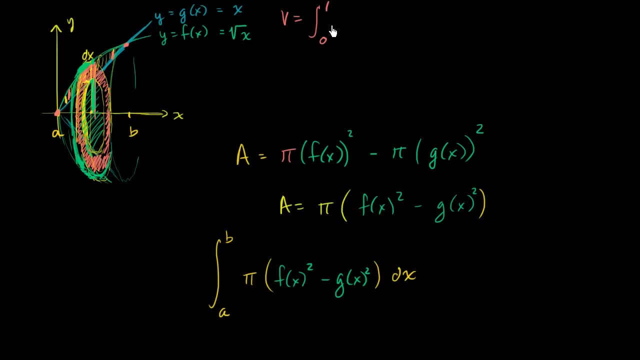 We saw that in the last video. Of pi times, what's f of x squared?